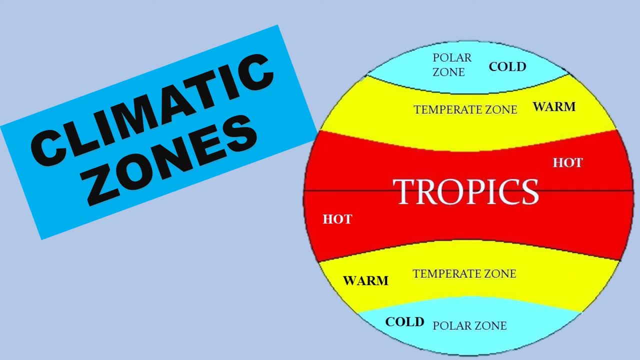 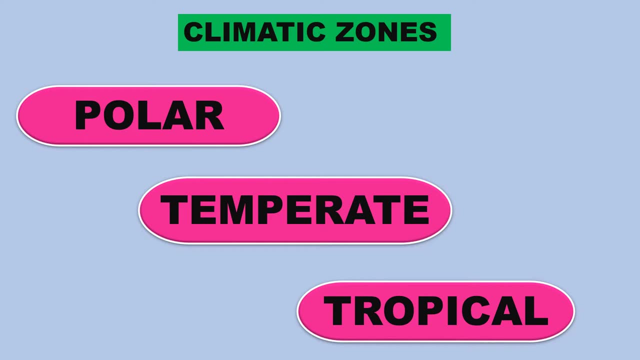 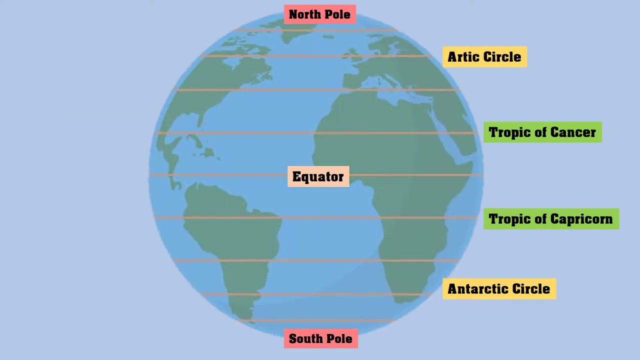 Hello everyone, welcome to another video. Today we look at climatic zones. Earth is divided into three main climatic zones. They are the polar zones, the temperate zones and the tropical zone. Each climatic zone is separated by lines of latitude. Let's learn more about these zones. 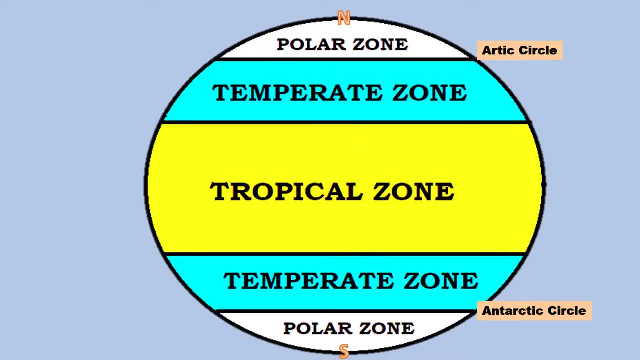 The polar zone. There are two polar zones on earth. One starts at the north pole and ends at the arctic circle, while the other starts from the south pole and ends at the antarctic circle. This is the coldest zone During summer. 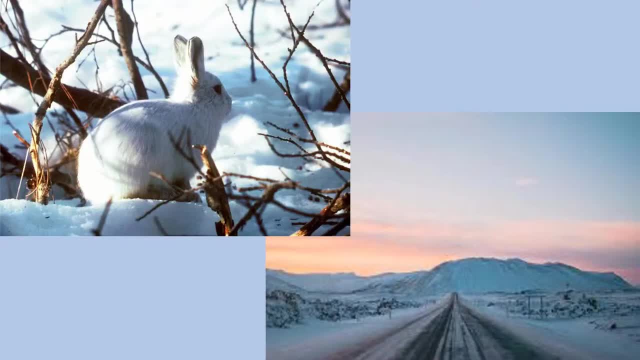 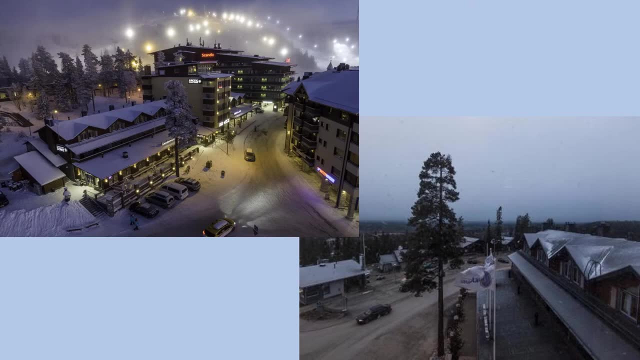 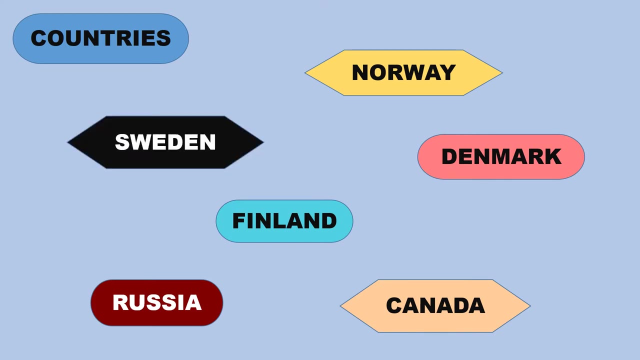 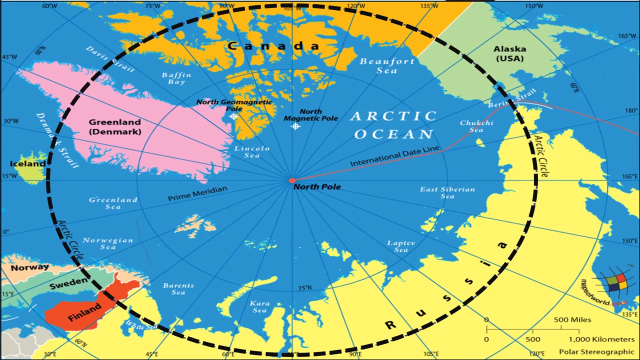 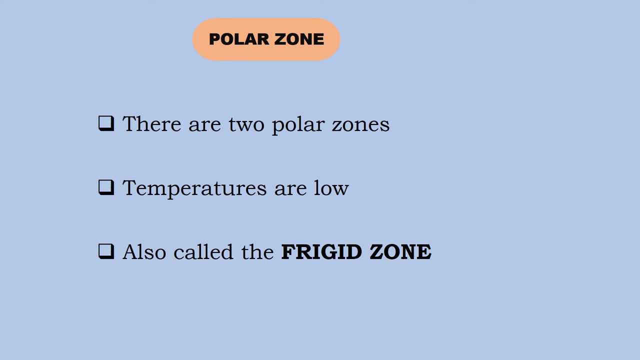 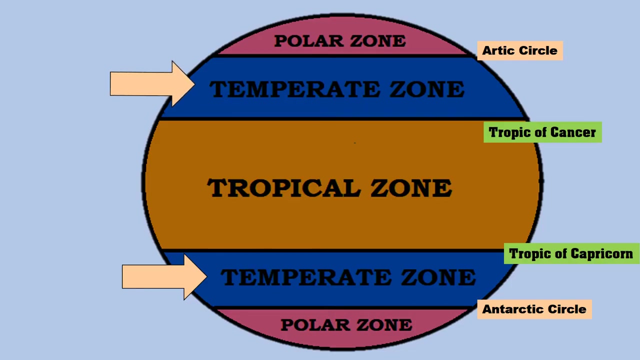 there is continuous daylight, while in winter there is continuous darkness. This zone is also called the frigid zone. Some countries that fall in the polar zones are Sweden, Norway, Denmark, Finland, Russia and Canada. The Temperate Zone. Earth also has two temperate zones: one to the north, between the Arctic Circle and the 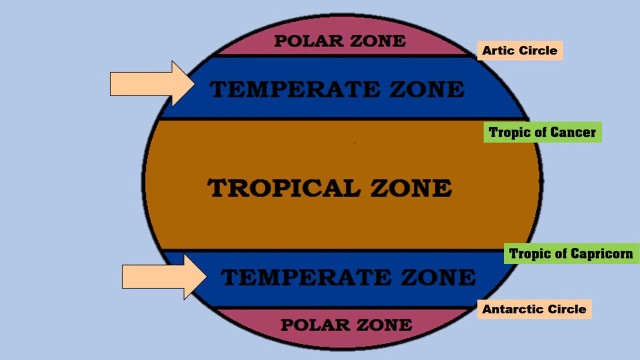 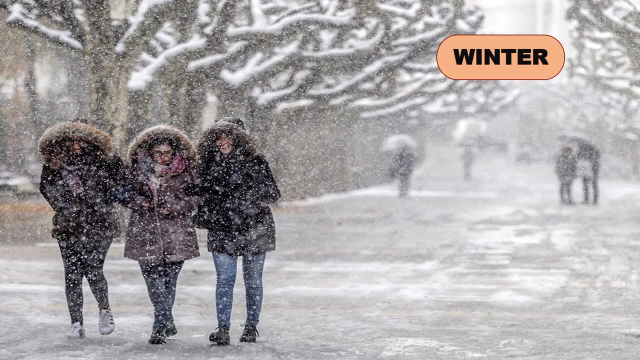 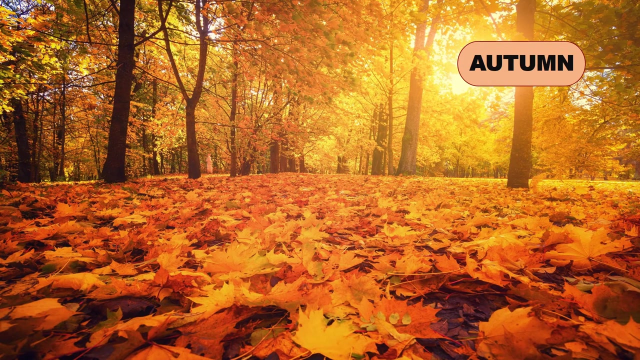 Tropic of Cancer and the other to the south, between the Antarctic Circle and the Tropic of Capricorn. This zone experiences long winters and short summers. There are four seasons in the temperate zone. They are winter, spring, autumn and summer. 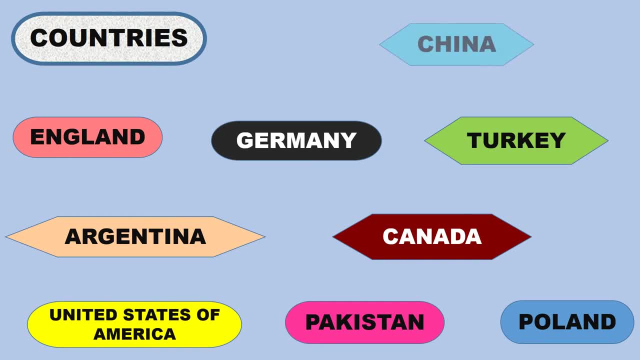 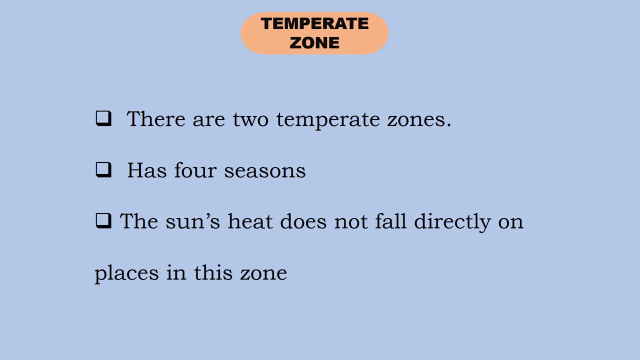 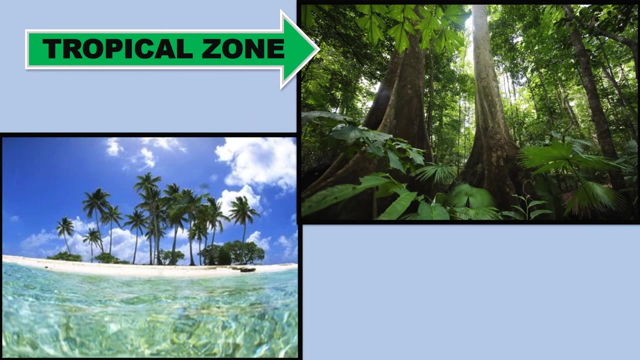 Some countries in the temperate zone are China, England, Germany, Turkey, Argentina, Canada, United States of America, Pakistan and Poland. The tropical zone: We will find the tropical zone between the Tropic of Cancer and the Tropic of Capricorn.